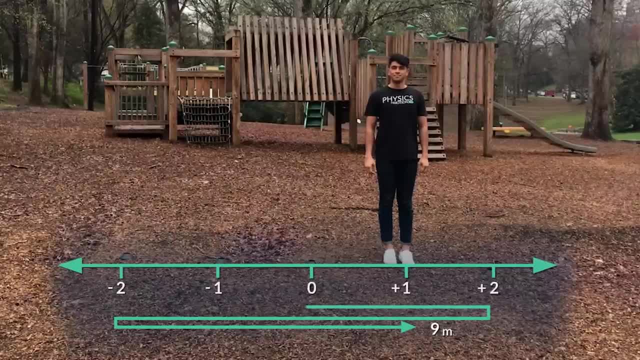 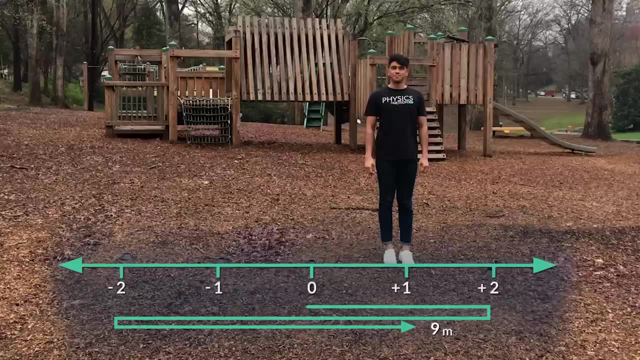 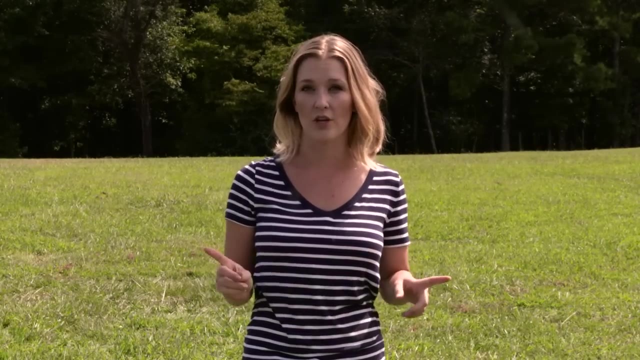 when measuring distance, the path he takes between an origin and destination matters. So, even though he ended up only one meter away from his origin, his total distance traveled is still nine meters. But what if Anzur didn't want to know the path he took throughout his journey, and only? 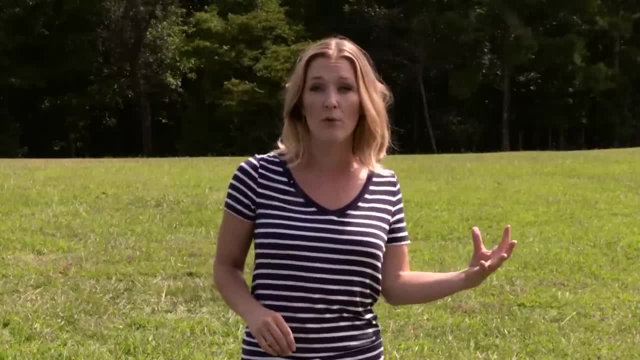 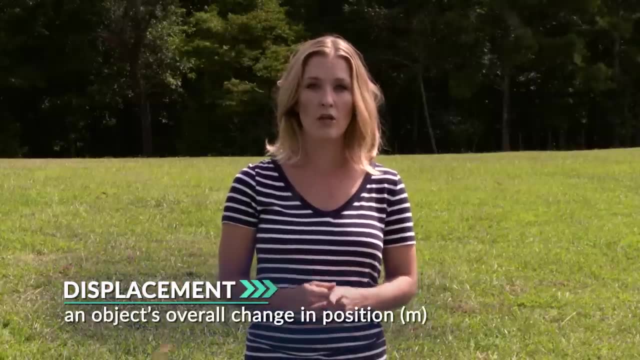 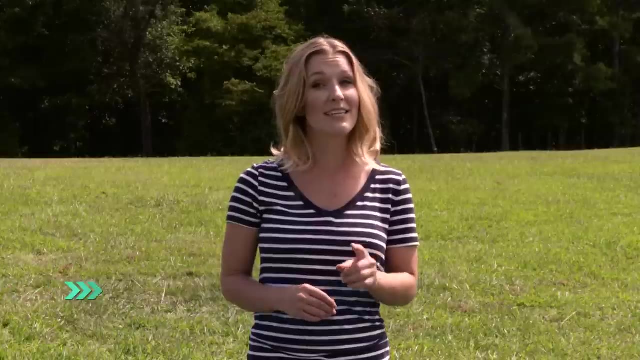 cared about the difference in meters between his starting point and ending point. That's where displacement comes in. Displacement is an object's overall change in position, Just like distance. the SI unit for displacement is meters. Displacement is a vector quantity. 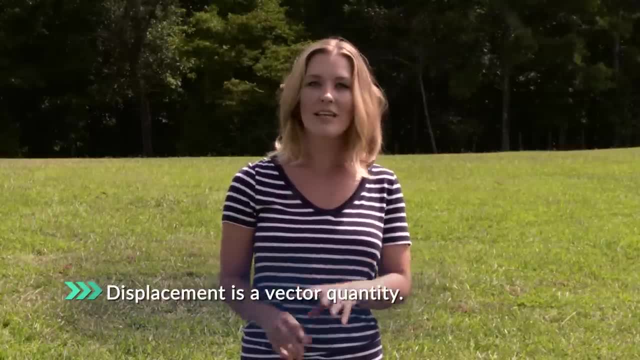 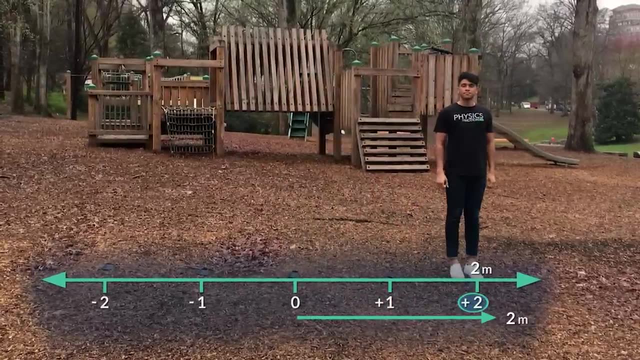 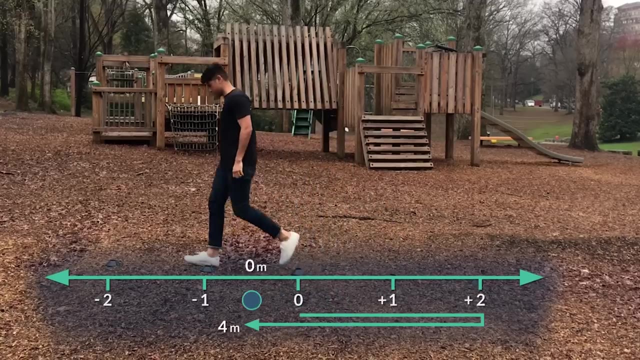 which means it has a magnitude and a direction. So let's go back to our number line. If Anzur moves two meters this way, the distance he moves is two meters, just like before, But his displacement is two meters to the right. Now if he moves four meters in the opposite, 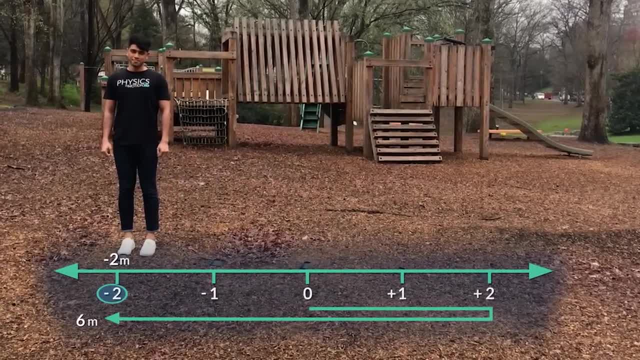 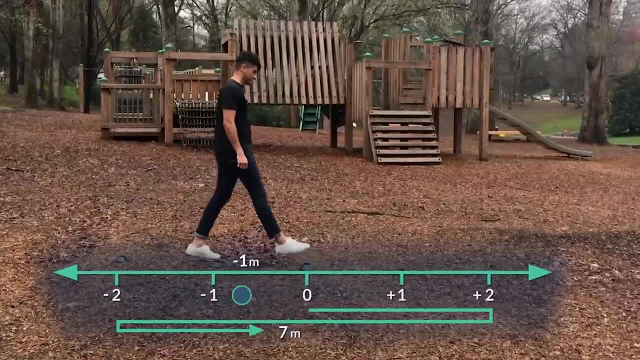 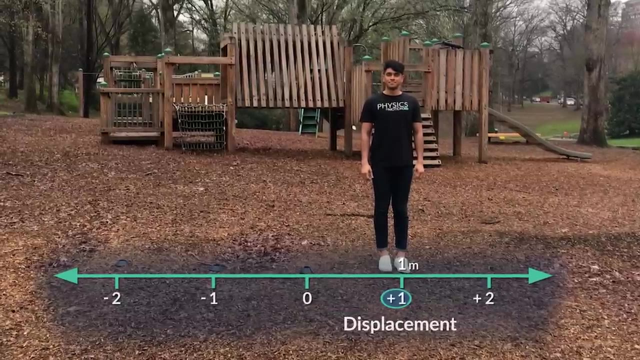 direction. the total distance he's traveled since starting is six meters. However, his displacement is negative two meters. So if he moves three meters to the right again, his distance adds up to nine meters, But his displacement for the whole journey is one. 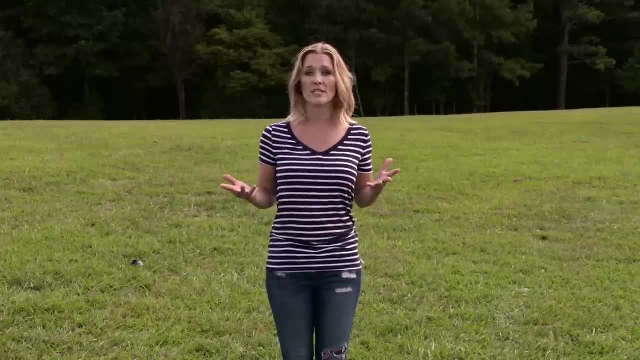 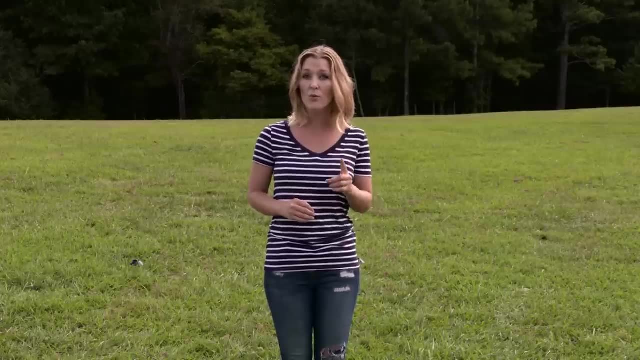 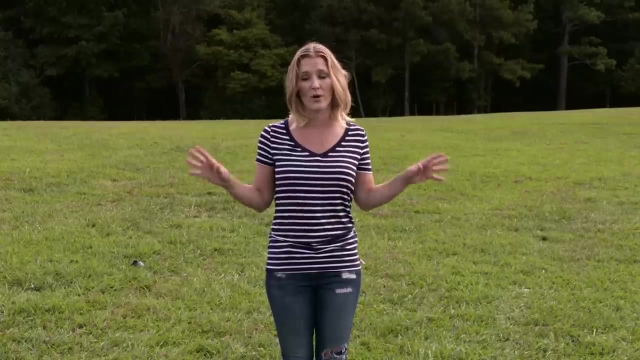 meter to the right. So why is that? We know our displacement is the difference in meters between our initial position and our final position. That means the route we took to get there doesn't matter. The only thing that matters is how far we are from the origin and in what direction. 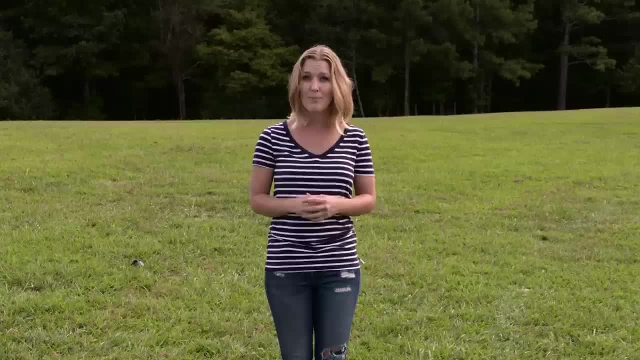 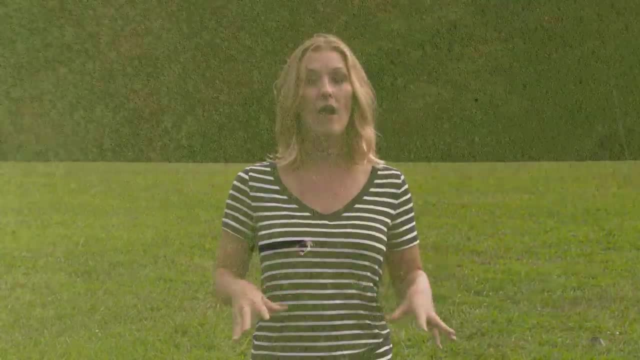 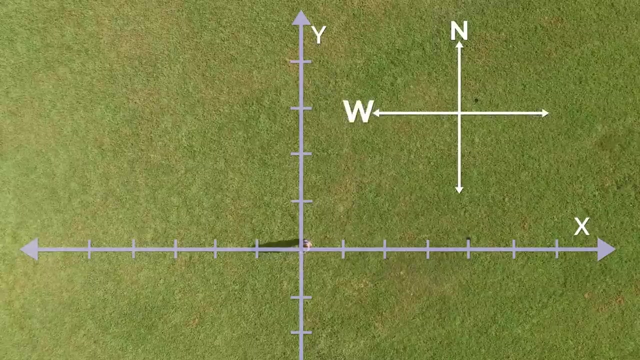 we ended up. So his distance was nine meters but his displacement was one meter to the right. But enough with number lines. Let me demonstrate using a grid. Where I'm standing right now is my starting point or my origin. On this grid, north is up, west is to the left, south is down and east is to the right. 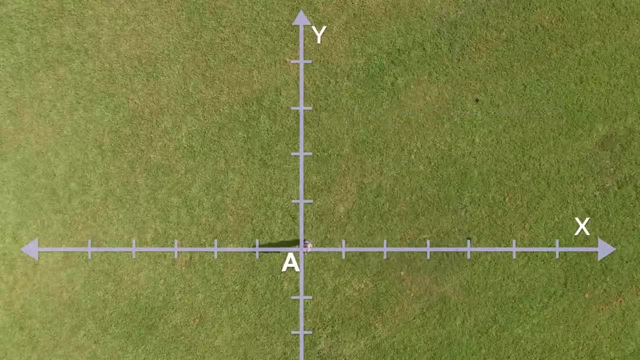 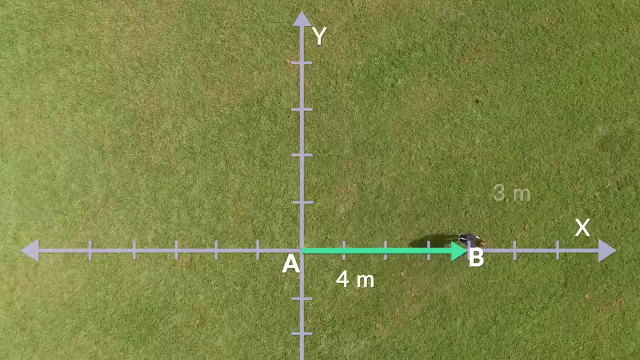 Let's call the origin point A on the grid. I'm going to move four meters to the right or eastward to what we can call point B. Next, I'm going to move three meters north to what we can call point C. 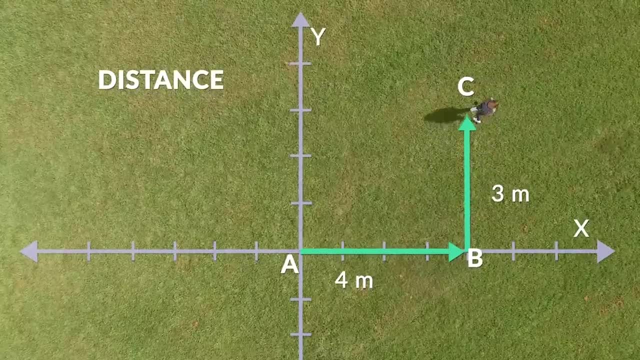 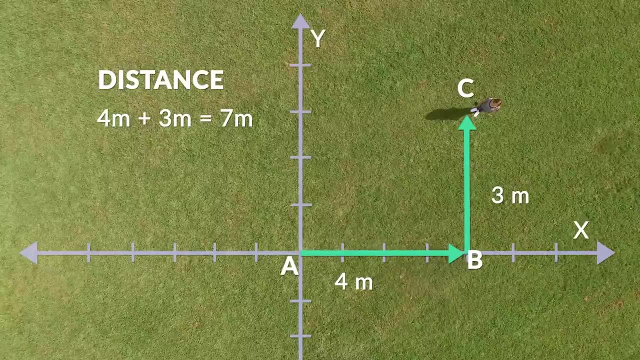 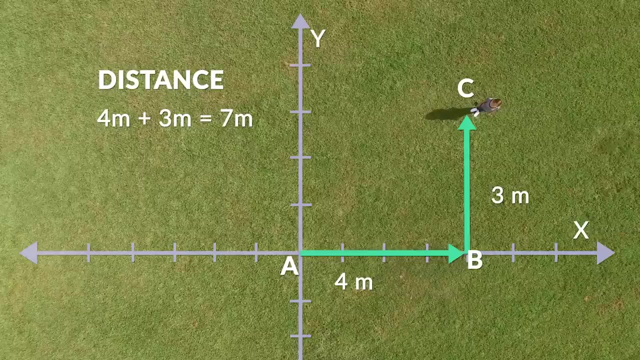 The total distance I traveled since I left point A is four meters plus three meters, which is a total of seven meters to get to point C. With distance, we only need to know the route that we took to go from our origin to our destination, But with displacement, we only need to know the origin and destination. and